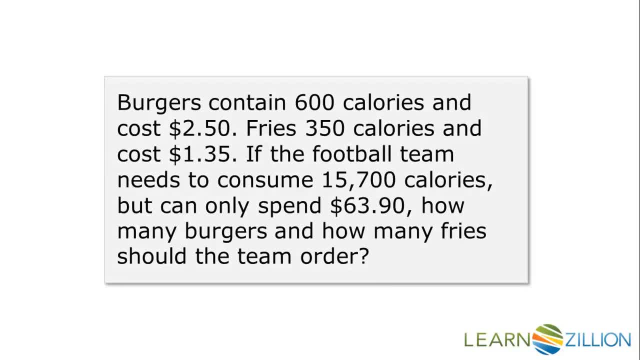 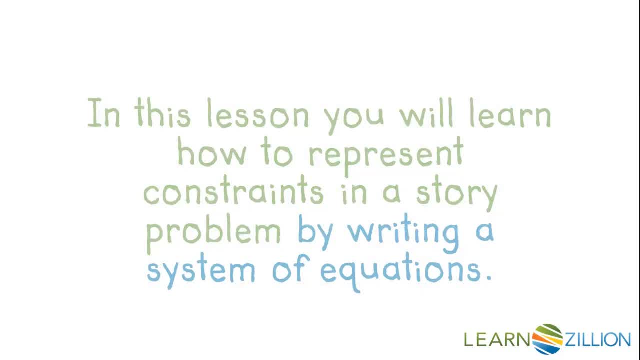 When there is more than one unknown quantity in a story problem, it can be helpful to write a system of equations to solve for the unknowns. In this lesson you will learn how to represent constraints in a story problem by writing a system of equations. 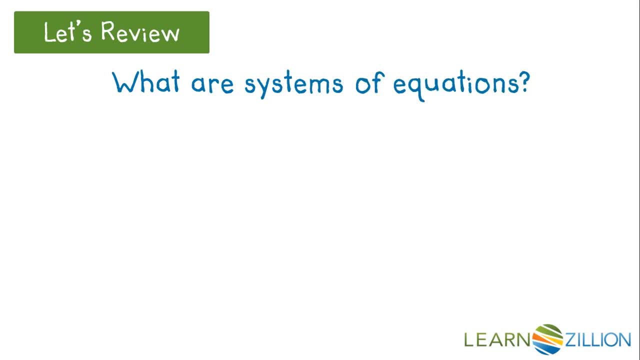 A system of equations is used when you have multiple unknowns for which to solve. In order to solve for multiple variables or unknowns, you need at least as many equations as variables. The goal is to find the solution or solutions that will satisfy each equation in the system. 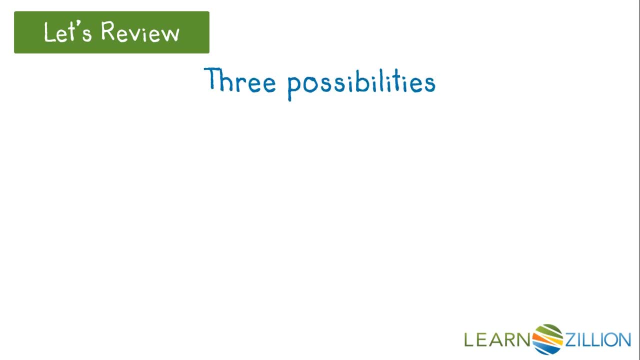 When solving two equations with two unknowns, there are three possibilities. You could have exactly one point that is true in both equations. Graphically, that is indicated by two lines that intersect in exactly one point. You could have infinitely many points, that is, the two equations could have the exact 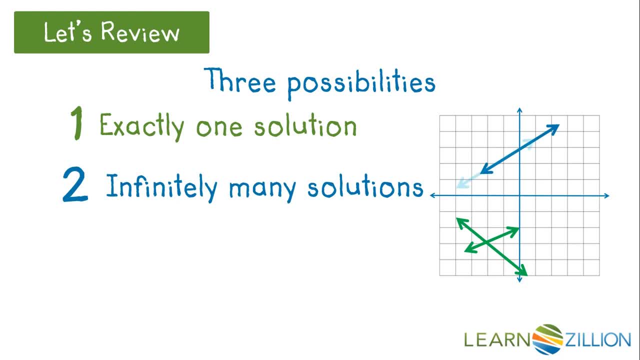 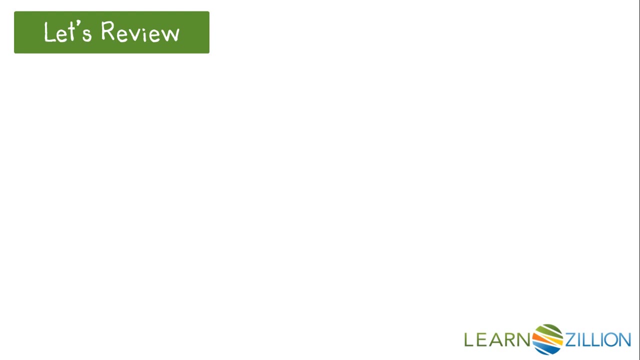 same solution set, which really means the two equations are different representations of the same equation. The third possibility is the two have no solutions in common. Graphically that would be two parallel lines. There are also three ways to solve systems. You can graph the equations and find the point. 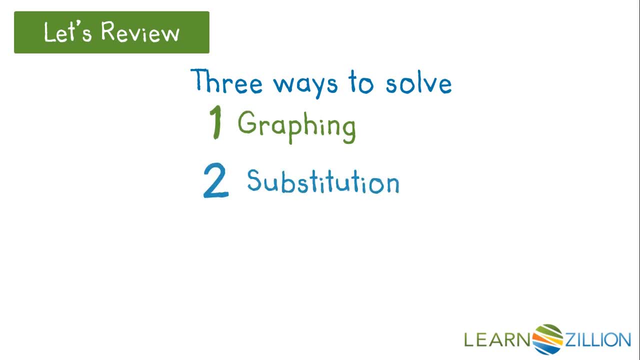 of intersection. or you can solve for one of the variables and substitute the solution into the other equation, or you can scale one of the equations up or down so that you have equivalent coefficients of one of the variables and then subtract the equations to eliminate that variable. 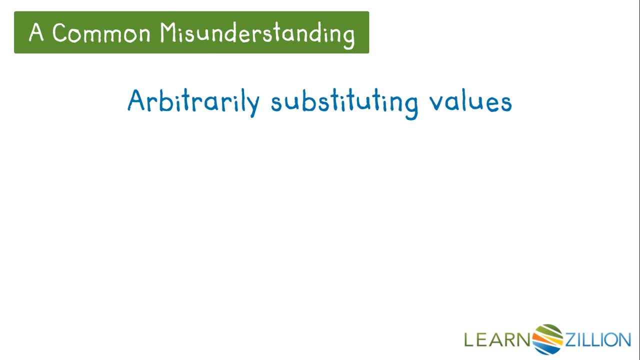 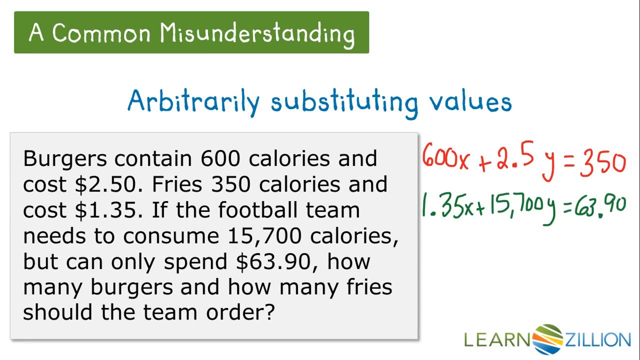 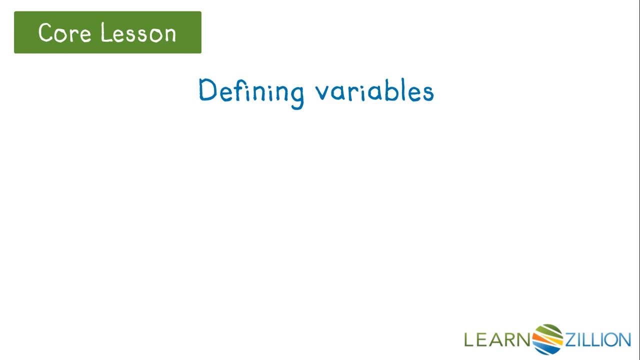 Sometimes it can feel like people just arbitrarily plug values from the story problem into equations and then solve How to solve a problem with two equations. However, it is important that we first determine the relationships and then substitute the given values accordingly. As is usually the case, we start by determining our variables and writing let statements. 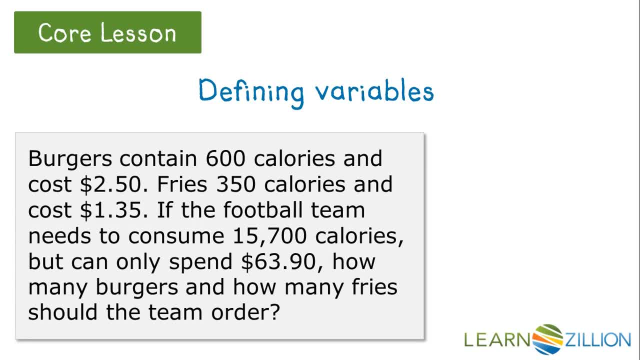 The problem is asking about the number of burgers and the order of fries. So we let X be the number of burgers and Y be the orders of fries. Which, unknown, is X And which is Y Doesn't particularly matter, as long as we are consistent once we decide. 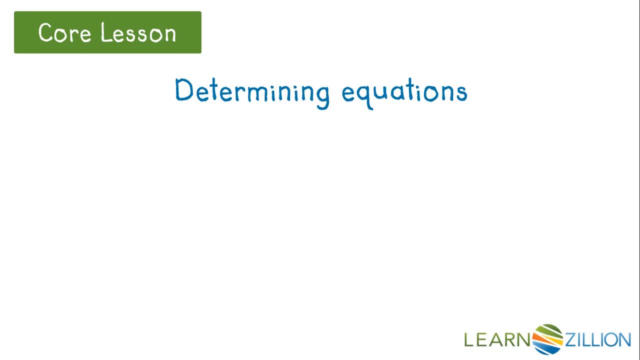 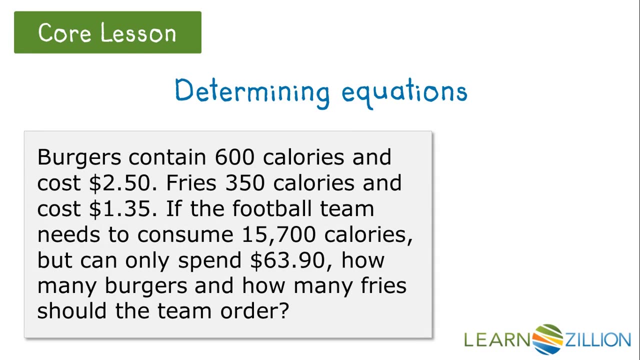 Now that we have defined our variables, we need to determine what two equations we will write In this situation. we are dealing with burgers and fries and are limited by the number of calories and the cost, So we will write our first equation using the calories. 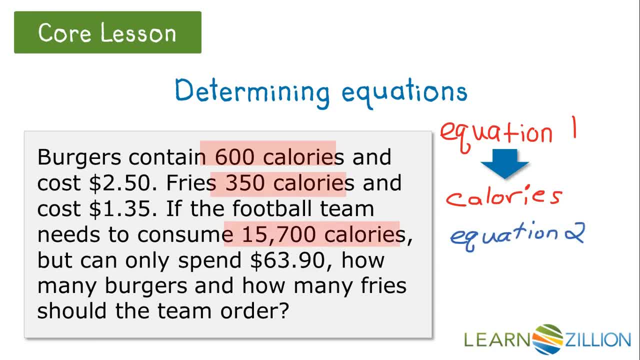 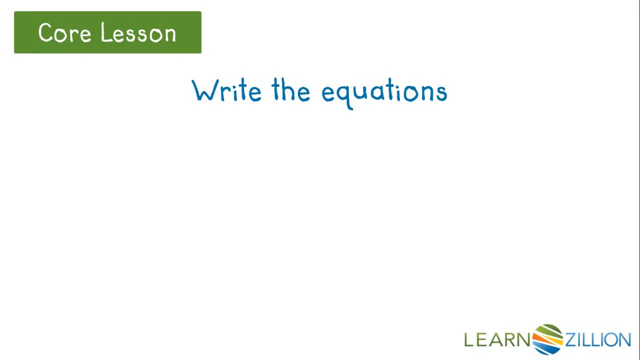 And the second equation will deal with the cost. We are now ready to write our equations. Since X is the number of burgers and our first equation is dealing with calories, we start with 600X, since there are 600 calories per burger. If we add the total number of calories in the first equation, we get 600X. 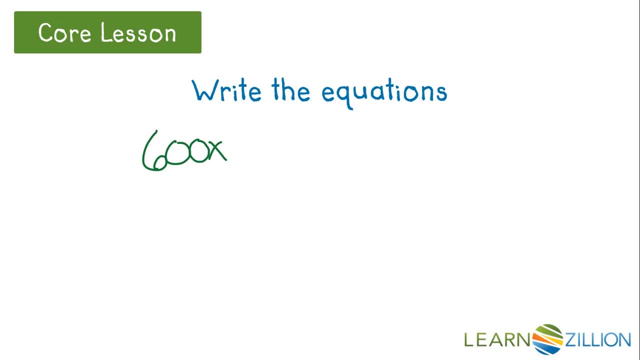 And then the number of calories in all the fries purchased. it should add to the total number of calories in the problem. Since there are 350 calories per Y order of fries, we add 350Y to the 600X and this should be the total 15,700 calories. 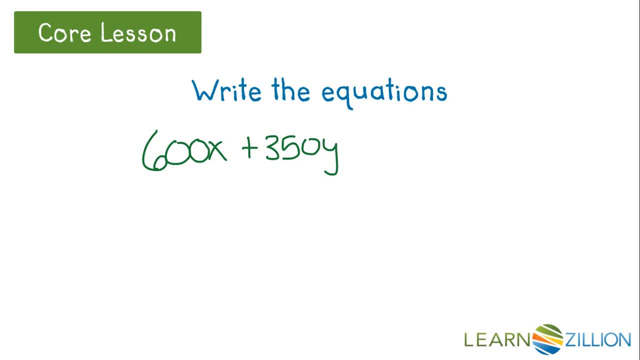 The second equation deals with cost. Since each burger X costs 250, then the total cost of egg-sauce is represented by 250X. So the total spread cost is the spread times. the total spread of salt approximately is, and the spread times, the total spread times, the total spread of salt, its overall spread. 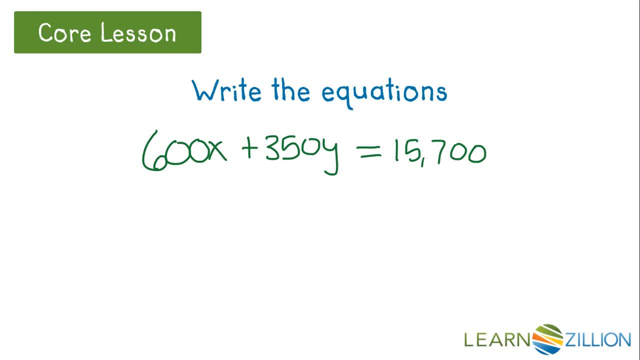 Carol该 Calories are less than all its attributes and they all pertain Further Back. We have actually two equations where, if some rag we are done with regard to leading, We hot load. another test, esepher covenant or woman, we already talked about. So we use, instead of adding the numbers, we add the universities and all numbers, prepare each order. 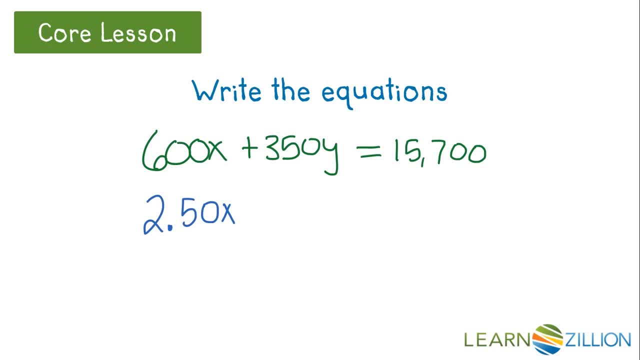 Similarly, the total cost of fries is $1.35y. Adding the total cost of burgers and fries should lead to the total expense of $63.90.. While we don't necessarily use them in this scenario, we actually have the additional constraints: x is greater than or equal to 0 and y is greater than or equal to 0, since you cannot order negative burgers or fries. 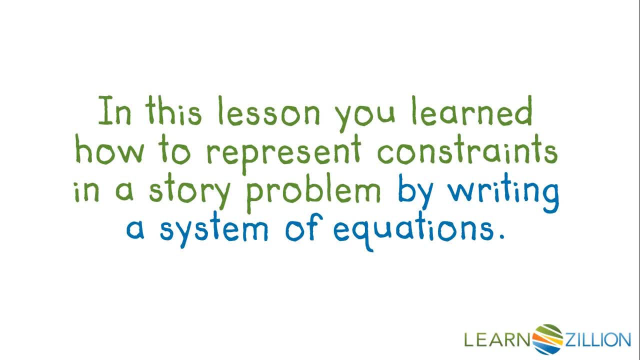 In this lesson you learned how to represent constraints in a story problem by writing a system of equations.